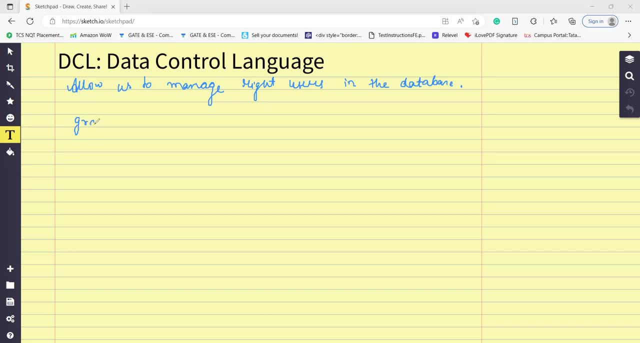 So these are the two commands that we use. First is grant and second is revoke. So grant is used to give the access, Revoke is used to, yeah, like to take the access back from that certain user. Okay, So like how we can do that. So, first of all, to assign any access, 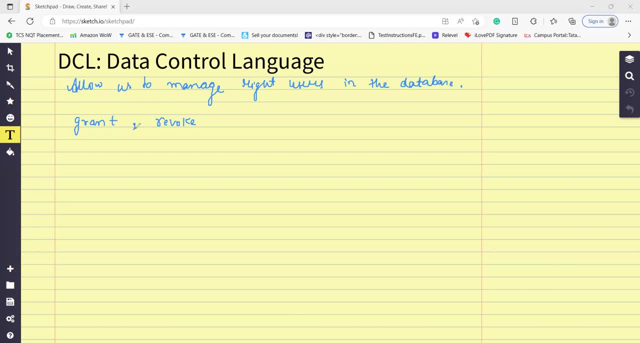 to a user, there should be a username that should be registered on that server. Let's say we have this local server, We are going to work on the workbench, So we have this local server, which is local host, but big, big companies, they have their own servers. 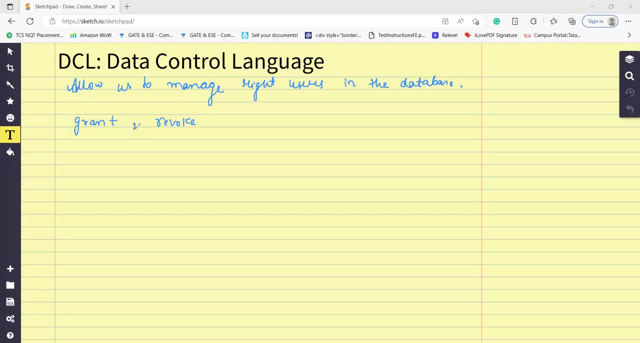 So they are going to register the user and they are going to provide the username And, according to that, they are going to provide access to it. Okay, Which is also called as permission: providing permission to the users. So let's try to understand how to do this. 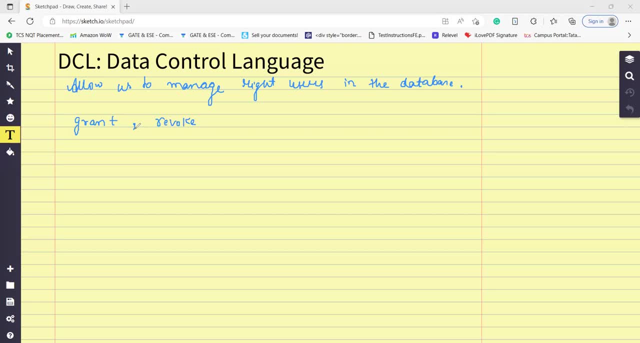 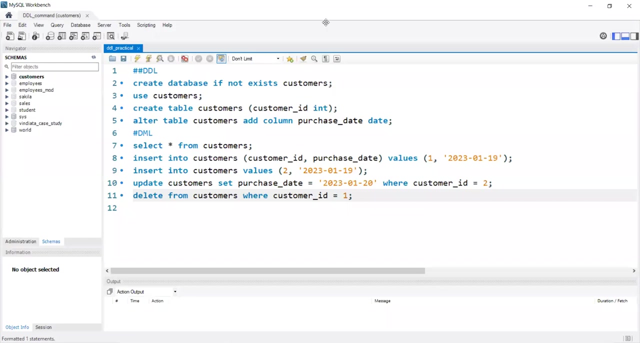 And in this class we are going to do the practical together, because then we will be able to understand that. Okay, So let's start with the practical directly. Okay, I will now use my workbench, Okay. Okay, So let's see what we are going to do here. So first of all, I have opened the same file. 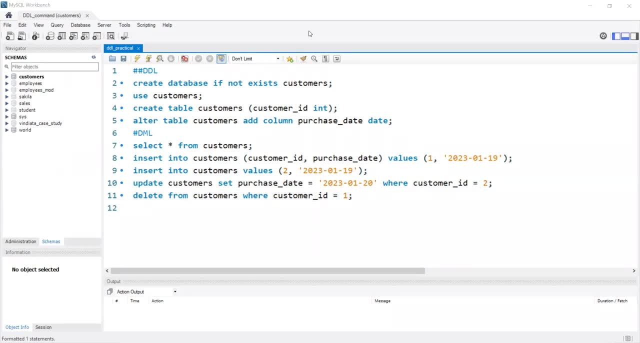 that we have- I mean same connection. We can see that we have used for DTM and DML commands, So we are going to see how to do it. So let's start First of all what I'm going to do. 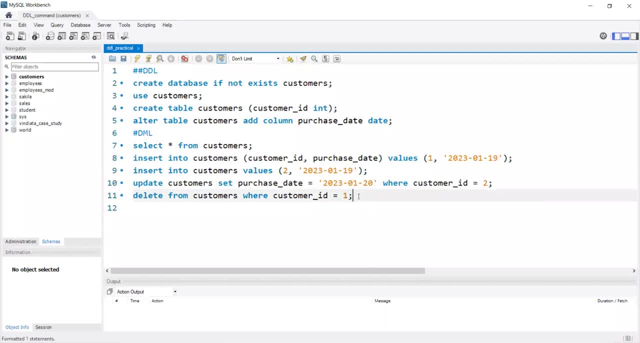 I will be making a user. We have to make a user and then we are going to provide access to that user. But before doing that, let me write it down that this is for this year. Let me increase the size so that we can see properly, And we have this customer's database. 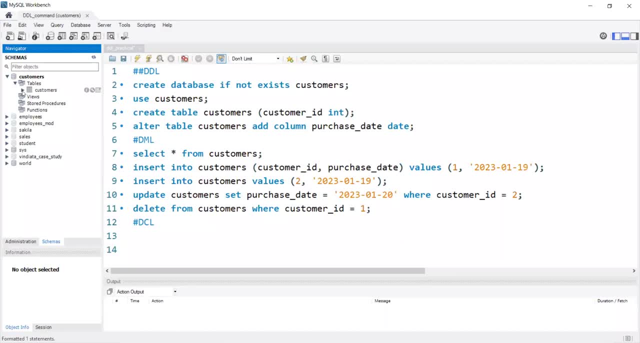 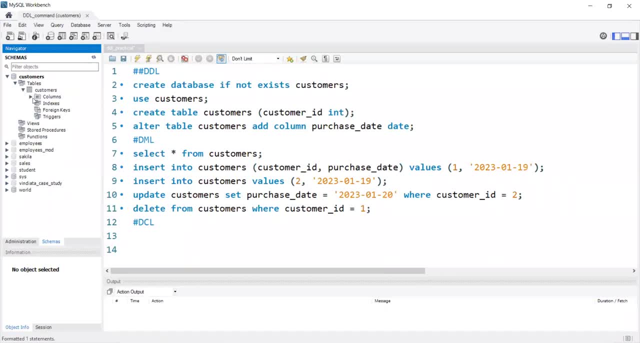 Let me do one thing: Let me add one more table in this. Okay, I'm going to add one more table, So I will just copy this line number four and I will paste it here and let's name this as sales And I'm going to name this as sale ID. So we have this table with one column. 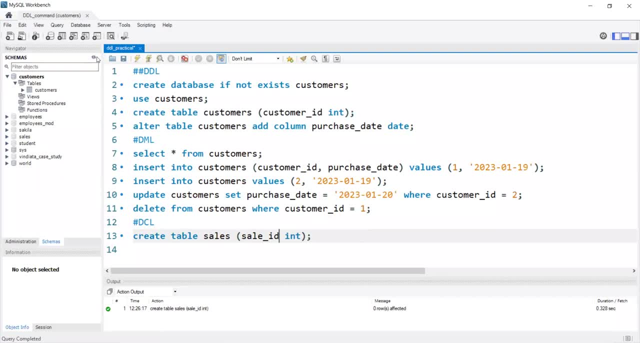 So let me run this. Yeah, it is created. Let me refresh this. Okay, So we have this table and we have this table with one column, So now we have two tables inside the customer's database. Okay, Simple, Let's go ahead. Now we are going to create a user. How to do that? 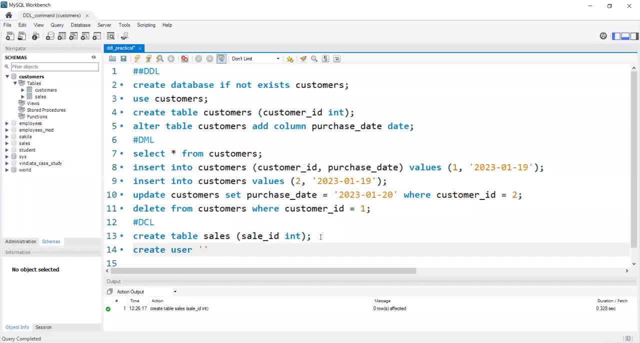 So we have to write on create. then we have to write on user. Now we have to give the name like to that user. So let's name, let's give that user as John. I'm going to write on John. Then we have to write on at and a server. We have this local host, so I will. 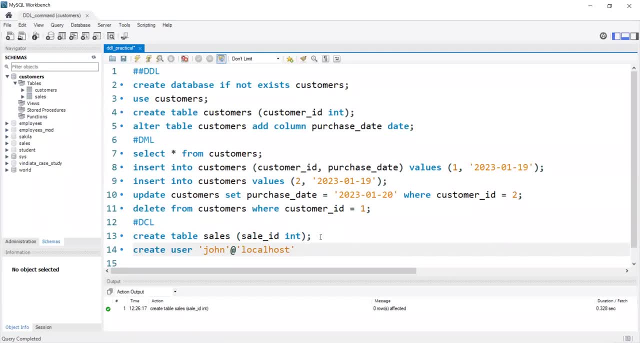 okay, and now we have to write this identify by. here we are going to provide the password. like every user will have their own password, so we have to provide the password. let's say I'm going to write down John only as password, or John123. okay, now let me execute this so. 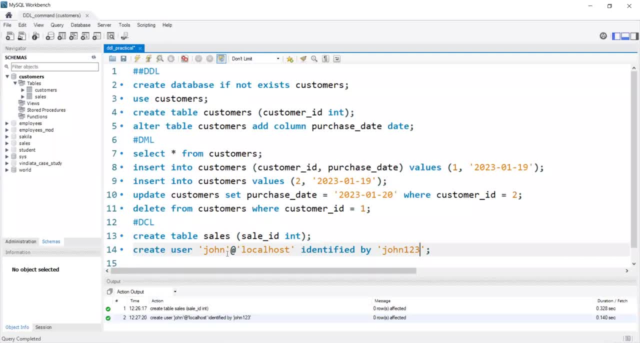 we have created a user named as John on our local server and the password is John123. let me copy this password because we are going to need that later now. so next, what we have to do. let me show you. so we have to now make a connection. okay, let's, let's talk about that. 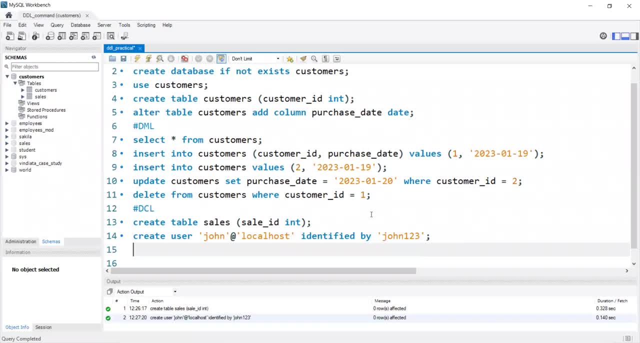 later. let's go ahead now. let's talk about this: like: what are the access we are going to provide to this user who is John? so to provide the access, we have to write down, grant. this is the case. then let's say, I only want to provide select. that means the user can only select and see. 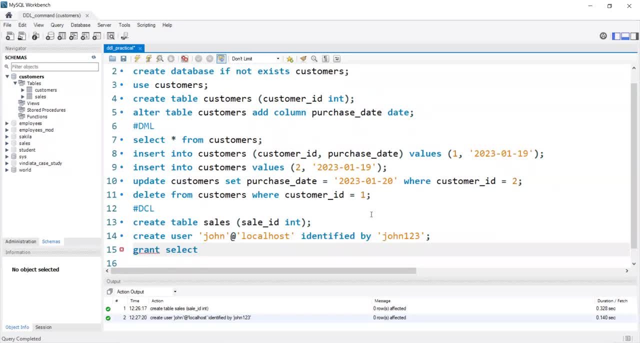 the database, how it is looking like and what are the things stored. the user cannot do anything else like insert, update, delete. nothing only serve on. now we have to provide on what, so I'm going to provide it on- on database which is named as customers and in that customers. 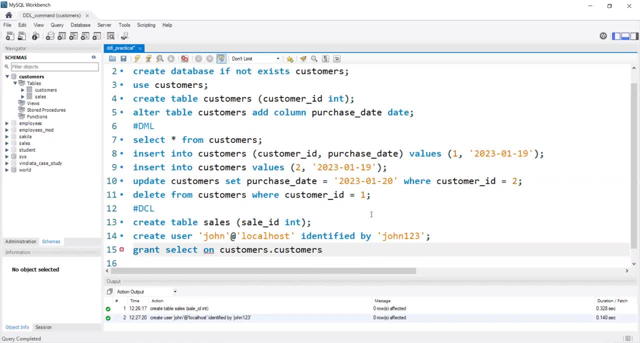 database, I will be only providing one table, which is customers. this is why I am providing a table which is called customers. so in this case, I'm going to provide a table which is: I created one more table that is called a sales. you will see what's the difference. okay to. 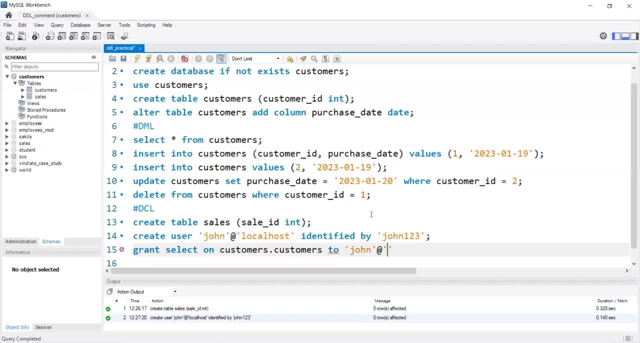 john at localhost. okay, fine, let me execute this also. yeah, this is done now, see, this is provided. we have provided the permission to john. now how to check whether they, whether this user, john, will able to access this or not? okay, so for that we have to create this user. now how to do that? so? 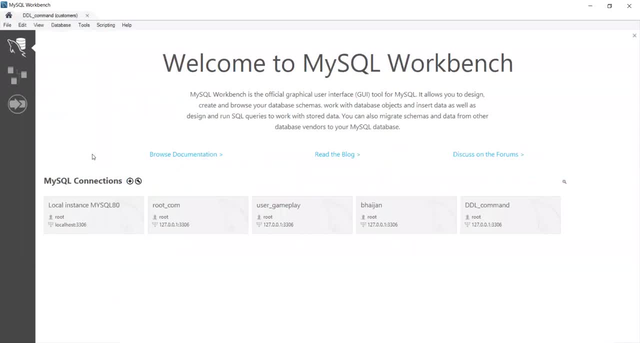 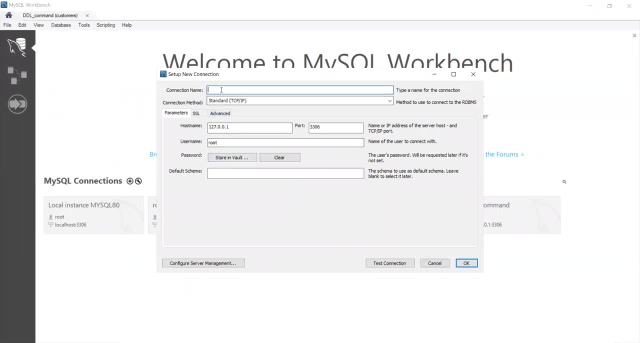 let's go back to our main page, home page, and here i will be clicking on mysql connections. okay, now see, we have to provide connection name. let's say john underscore. you can give any name. now we have to change the username. right, because the username is john, right? so be careful of that. 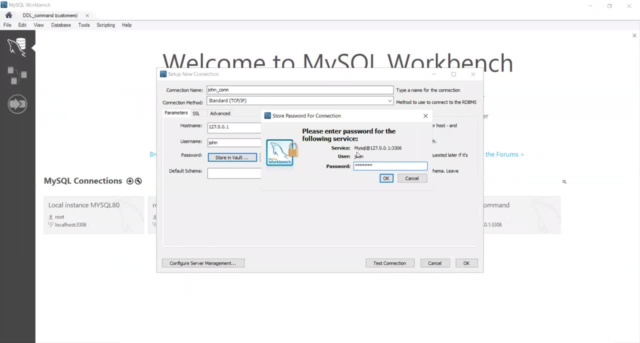 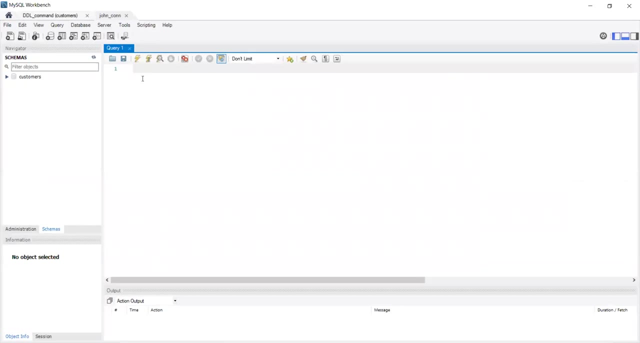 then password. so the password is john123, so i will. i copied that password, so i paste it here. now i'm going to click on ok and then i will click on ok and then i will open this connection. okay, so now let's try to check whether this is actually working or not. 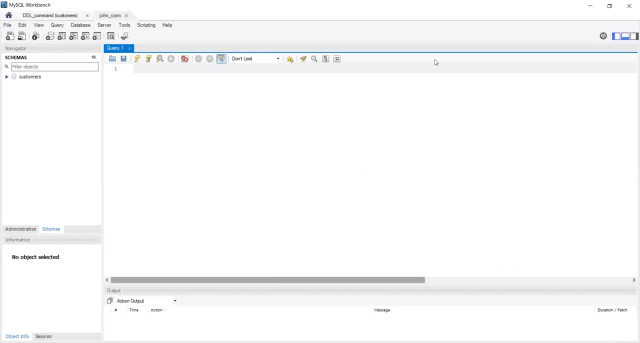 so, yes, it is working. now let me show you how. because if you see here: uh see, only customer database is visible and inside that john has access to table customers. only see, we created two tables- customers and sales- but we mentioned that john will only have access on customer database. 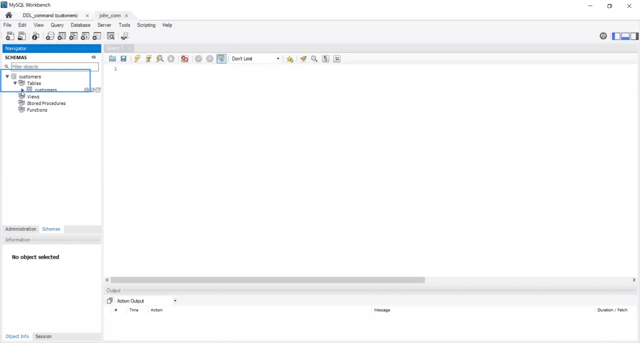 and customer table only. so only customer table is visible, okay, and the columns, which is customer id and purchase date. everything is fine till here. now let's try to write that. let's try to see whether john is able to use select command or not. so i will be writing select. let me increase the size. 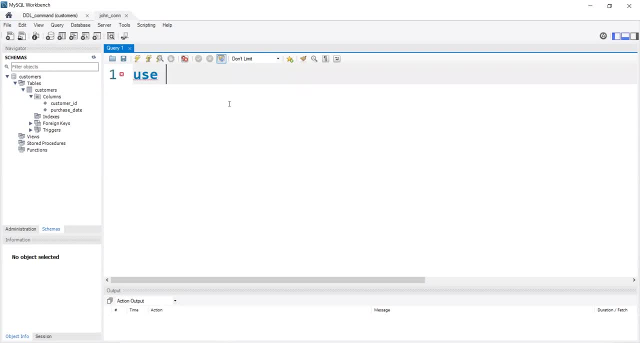 first, i have to mention that i want to use this database, that is, customers. okay, let me execute this. yeah, this is done. then i will be using select command, select star from customers. okay, let's see. yeah, we are getting this. this is what we did in the last uh dml video, so, if you remember, this is what wins on. 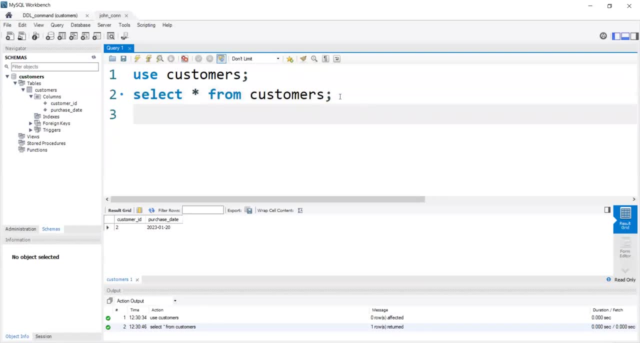 now let me try to use different query, uh, which is not about Desktop distinguish and select. let's say i want to use update or delete. let's use delete. delete from what customers? i want to delete all the data? okay, i will execute this. not see, i do not have access. 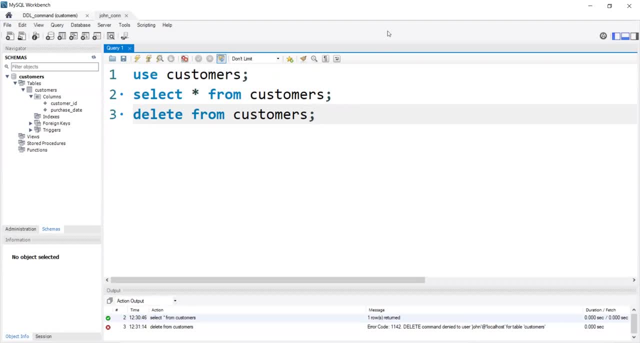 see, see, this query do not get executed. if you see, here i am getting that this is not run successfully. why? because the access is denied to user john on this table. because we provided only select as the permission right. so this is why we provide permission to the users. 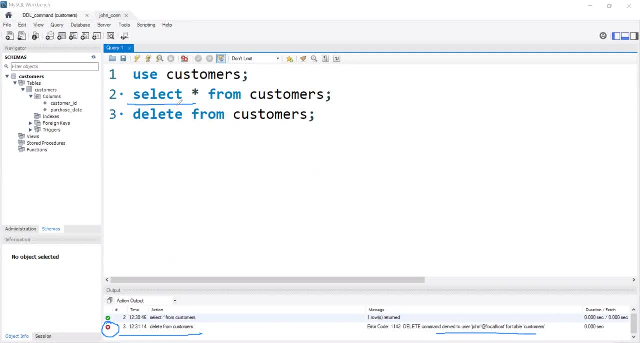 so that they do not, by mistake, delete everything or make any change to our database, because there are so many important information stored. so if there are going to be any small change, that will create a big problem. okay, so this is how we do it. now. let's say that. okay, i. 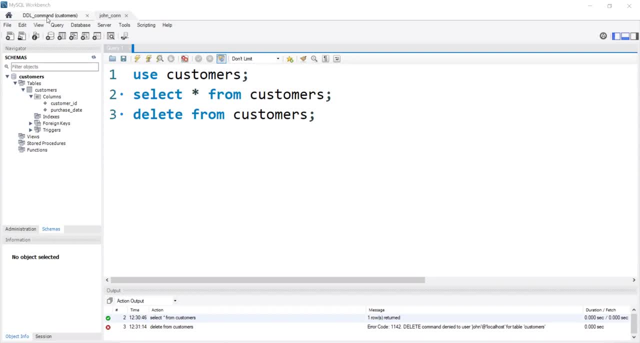 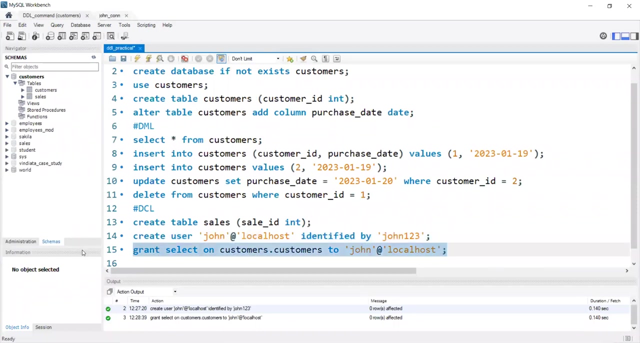 want to provide other access, other permissions to john. let's say that john is now very much stable and he has command and now he is able to manage our database. so how to do that? so let's go back here and i will copy this line, because we have to kind of copy this line. 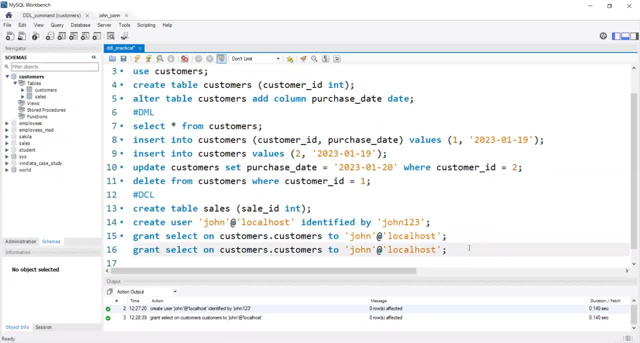 but use the same thing. i will be pasting it here. and let's say that i want to grant every permission to john, so i will be writing grant on on customer, customer. so let's say that we want to grant permission on every table that is present inside customer database. 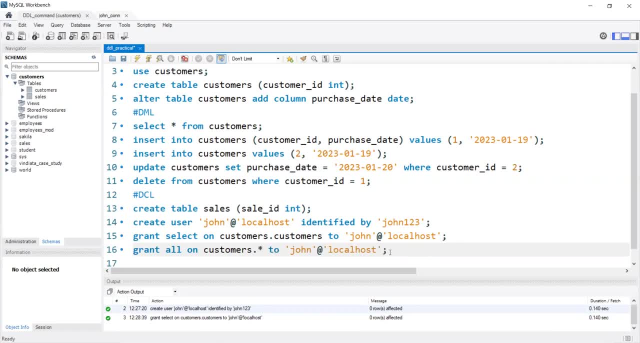 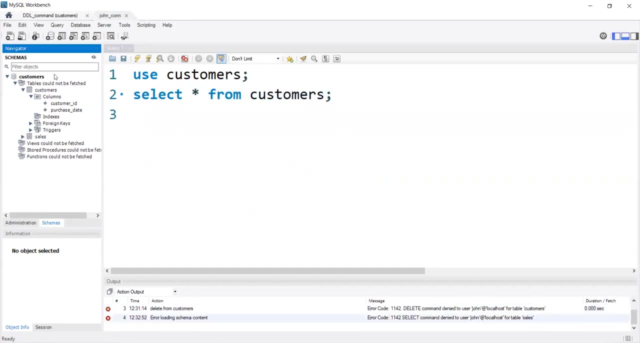 so again, we have to write on star. okay, and that's it. let's execute this query. yeah, it is done. now let's go back and i will delete this query. okay, so now let's go back and i will delete this one. okay, a problem. now let me execute this and let's see whether john 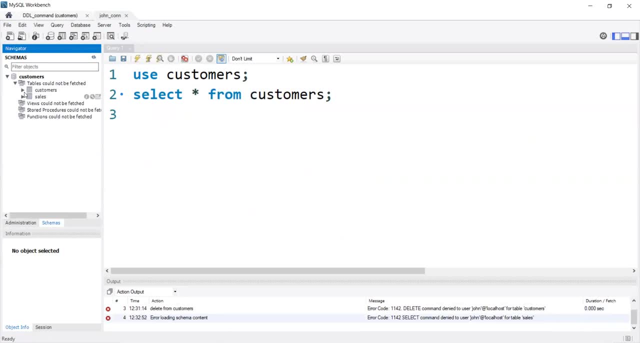 is able to see the tables or not. which is sales table? yes, john is able to now see sales table. see, right, so this is how we provide the access and now john will be able to do other uh query also like update, delete, truncate, everything. okay, so yeah, this is how we do. 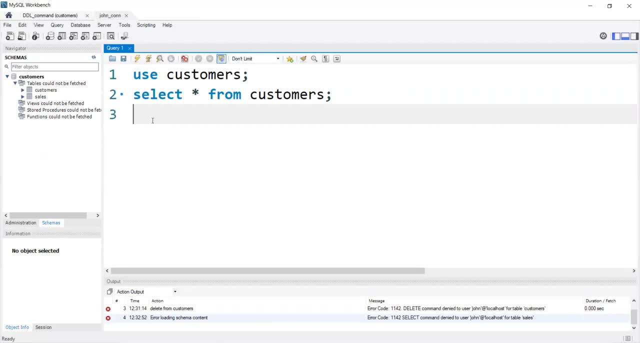 it. now let's talk about the report, so that's it. okay. so revoke is just opposite of craft, okay? so we take all those things that we have provided to the particular user. so how to write it? so let's go back to our code, and here we are going to again. 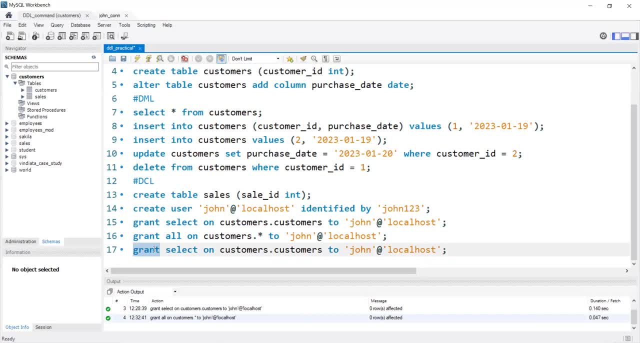 i'm going to take the same thing, i'm going to paste and i will be writing: review, revoke select on customer customer. we have to change to the from okay, so what will happen? so that john will not be able to use select on customer table of the customer database. 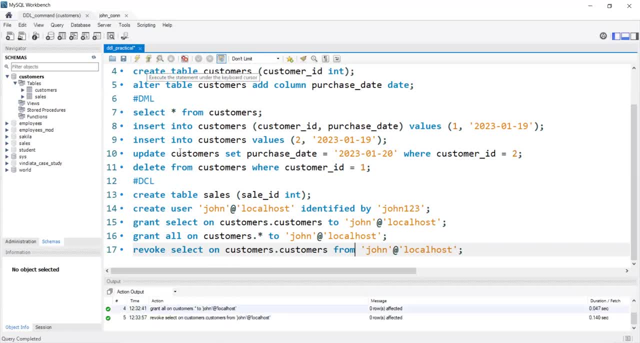 okay, this is what the meaning is, so i'm taking the access from him and see this query executed successfully. so this is how we use grant and remove, because different users have different access. so, according to the name of the problem, it will be used as pre-progress for each previous. 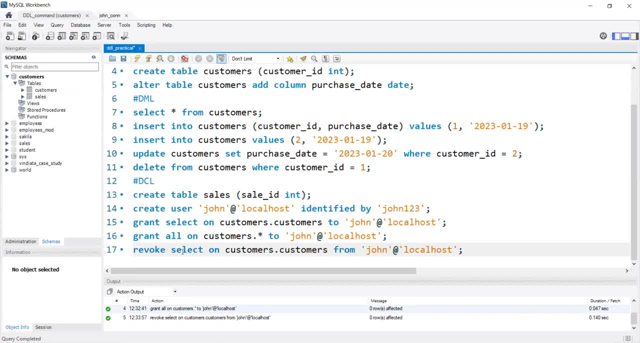 to that. you have to provide them the permission, okay, so that there will be no problem in your database. okay, that's it about grant and remote. so if you have any doubt, you can ask me in the comments. but if i say they are not used that much because, uh, right now we don't have to worry about 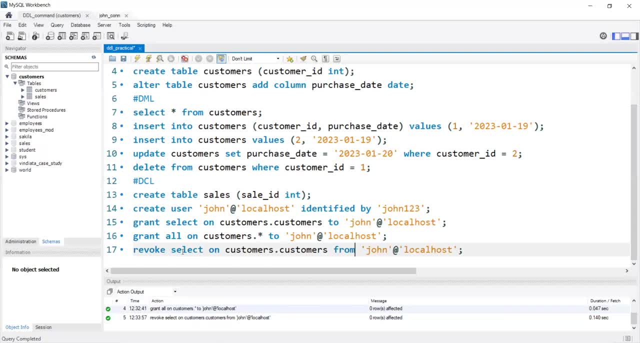 this, but still, it's good to have an idea about it. so yeah again, if you have any questions, you can always ask. so that's it from my side. have a nice day, take care. bye you.